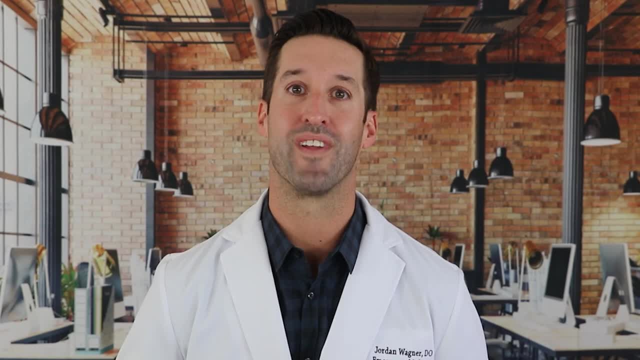 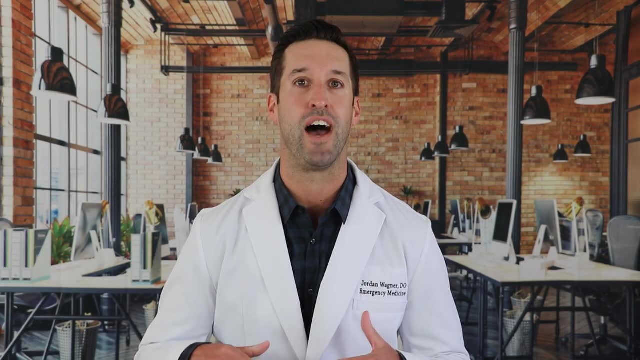 I wanna get huge for the summer. It can't be that bad right? Well, not exactly. Some steroids could have major health consequences on your body that you definitely should know about, and I'll go into all of that. But first things first. what the heck are steroids? 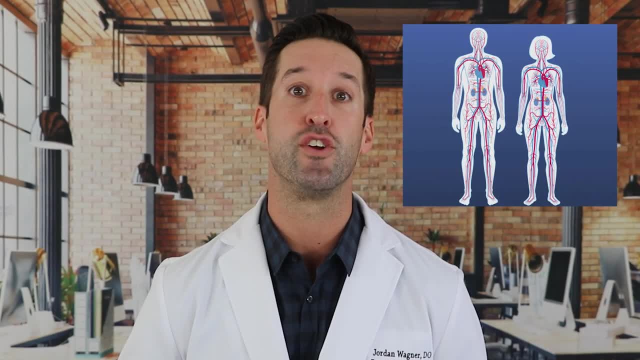 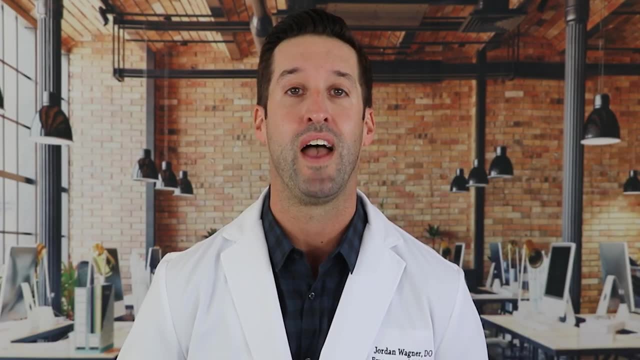 On a very basic level, steroids are chemicals, often hormones, that your body makes naturally. They help your organs, tissues and cells do their jobs and you need a healthy balance of them to grow and for other various processes in your body. But this term steroid can also refer. 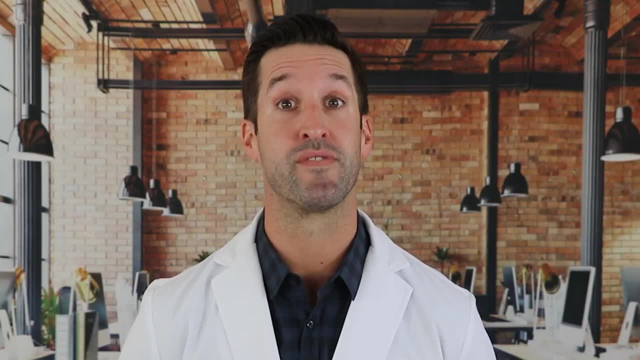 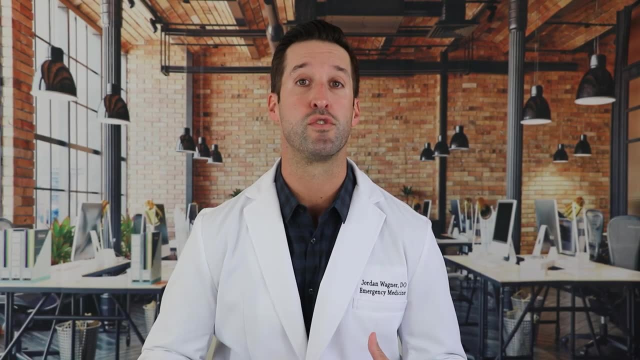 to manmade substances as well. There are two main types of steroids. The first are corticosteroids. Corticosteroids are a class of drug that lowers inflammation in the body. They also reduce immune system activity, ease swelling, itching, redness and allergic reactions. 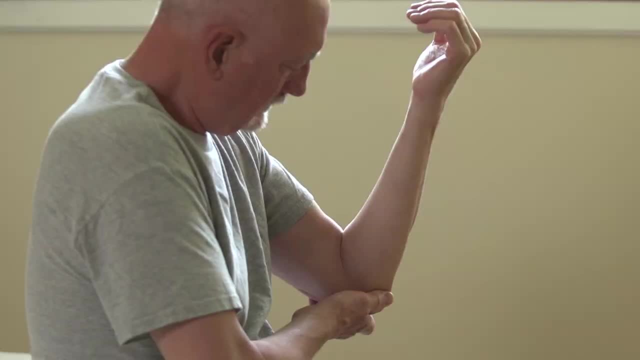 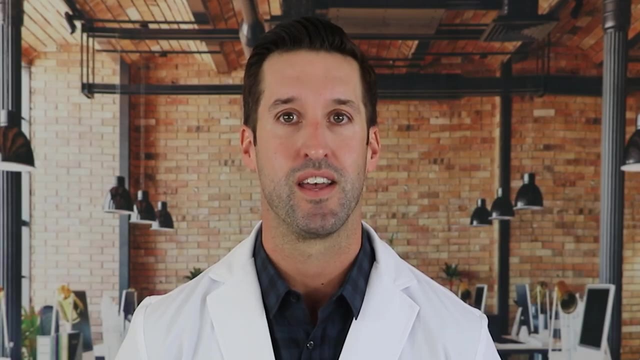 Doctors like myself often prescribe them to help treat diseases like arthritis in the knees, elbows or for asthma, And these corticosteroids have legitimate medical uses, But these are not, I repeat, not the steroids that you're trying to take to get big in the gym. 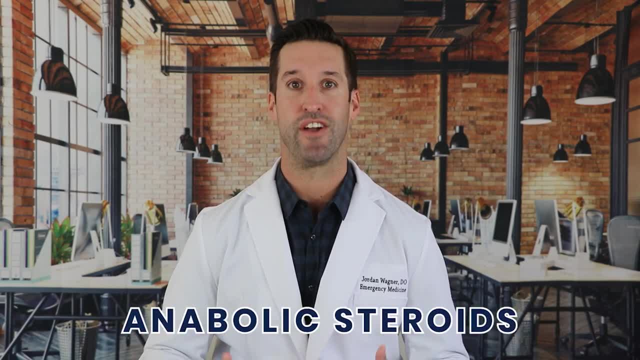 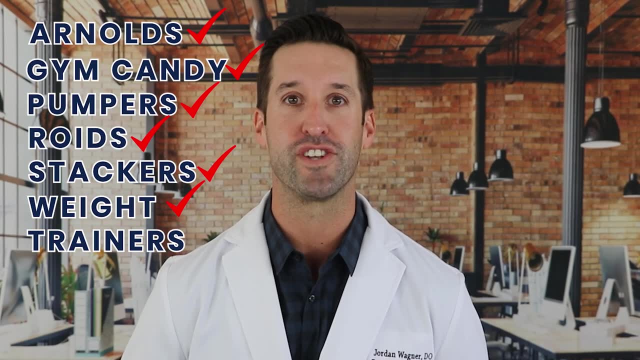 Those are the second type of steroid called anabolic androgenic steroids, often called slang terms like Arnold's gym candy pumpers, roids stackers, weight trainers and juice in certain fitness circles. Anabolic steroids are synthetic substances. 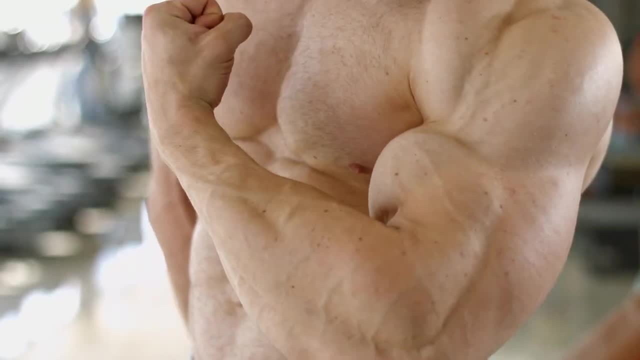 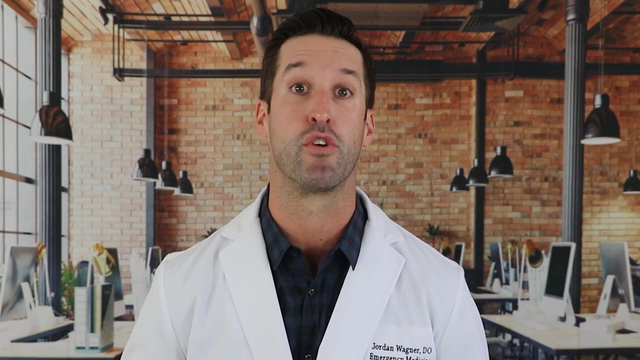 similar to the male sex hormone, testosterone. They work by stimulating muscle tissue to grow and bulk up in response to training, by mimicking the effect of naturally produced testosterone in the body. These types of steroids can remain in the body anywhere from a couple days to about a year. 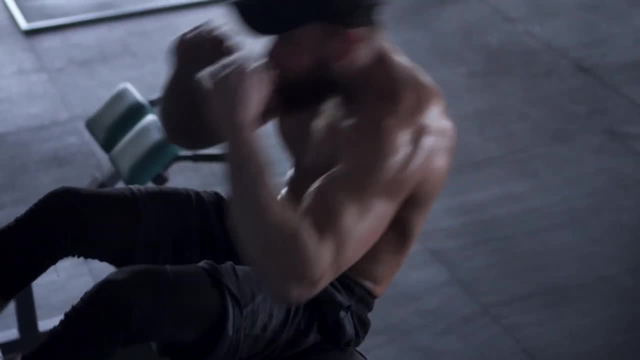 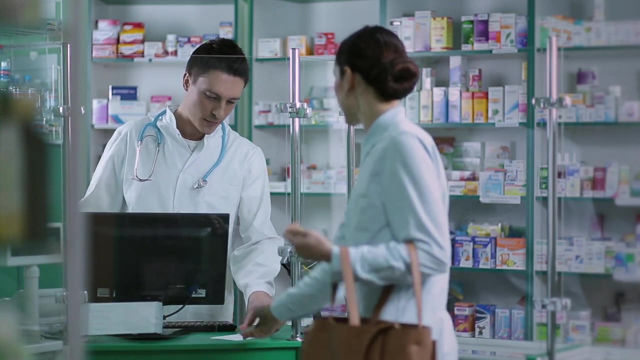 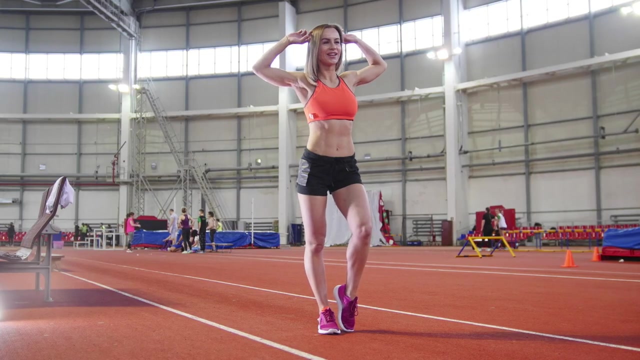 And they have become popular because they improve endurance, strength and muscle mass. These type of steroids can be prescribed for delayed puberty or for medical conditions that lead to muscle loss, such as cancer or AIDS, But doctors rarely ever prescribe anabolic steroids to young, healthy individuals to help them build muscles. 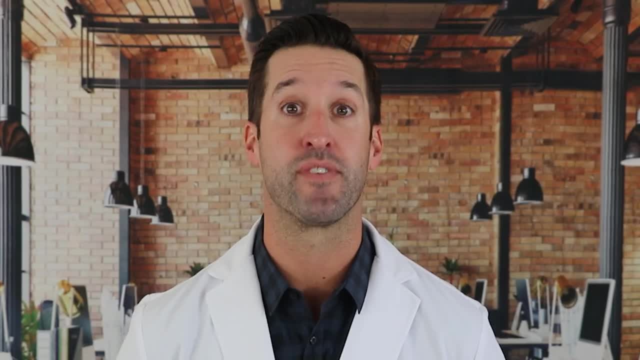 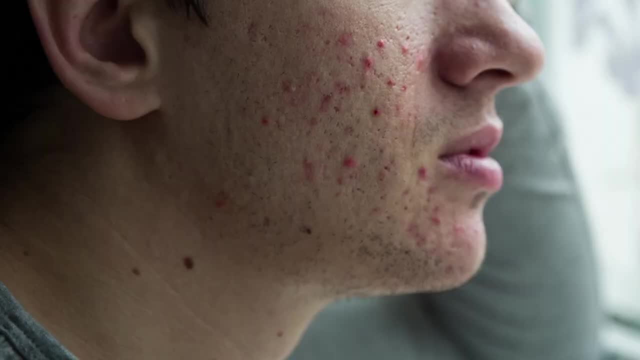 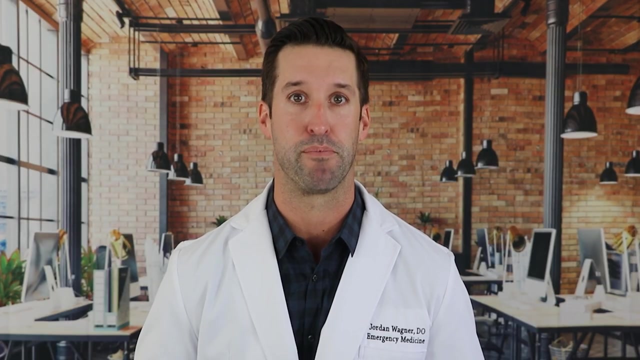 And without a prescription from a doctor, these types of steroids are illegal. All right. what are the common side effects of taking anabolic substances specifically, Aside from the small effects of increased acne and hair loss? when somebody abuses steroids medically, gender mix-ups happen. What I mean by this is men can grow breasts, experience shrunken testicles and reduced sperm count. Women, on the other hand, who take anabolic steroids, can grow beards, experience reduced breast size and experience deepening of their voice. 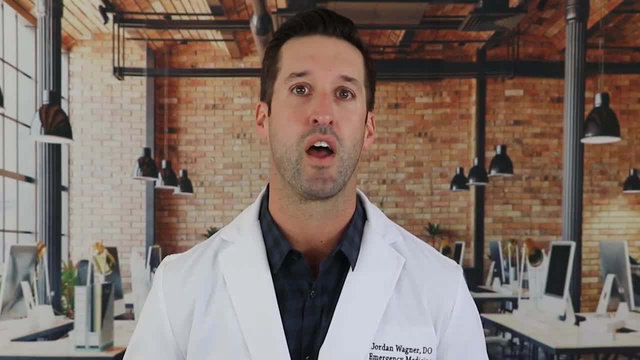 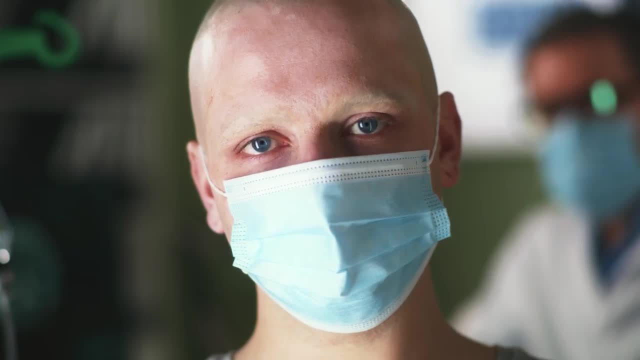 But these are not the only side effects. Steroids have major life-threatening effects as well. There are reports of an increased risk of developing liver cancer in the body. And if you don't develop cancer, some steroids are known to cause tumors that form in your liver, called hepatic adenomas. 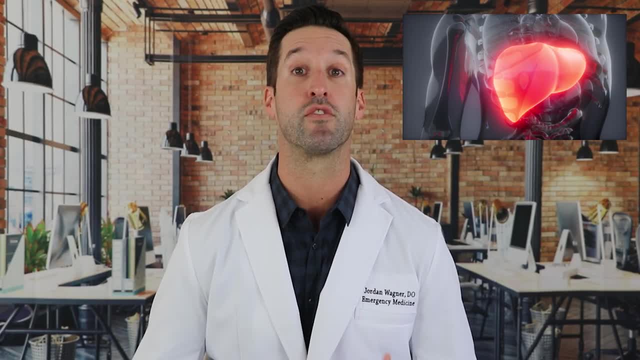 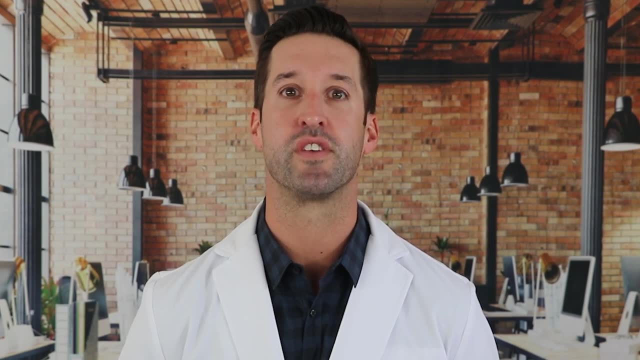 Although these tumors are not cancerous, they can rupture and cause serious bleeding in the liver. Your liver isn't the only organ that can be at risk either. The use of anabolic androgenic steroids is associated with compromised heart pumping and atherosclerotic plaque. meaning you could be at an increased risk for coronary artery disease and left ventricular dysfunction. Together, these effects can reduce the supply of oxygenated blood to the heart and from the heart to your arteries. Not to mention, these are the most common side effects of anabolic steroids. Not to mention high blood pressure, increased levels of bad cholesterol, mood swings, aggressive behavior, testicular atrophy, aka shrinking of your testicles, lowered sperm count and infertility, and many, many more other serious side effects. In other words, steroids throw your body way out of whack. 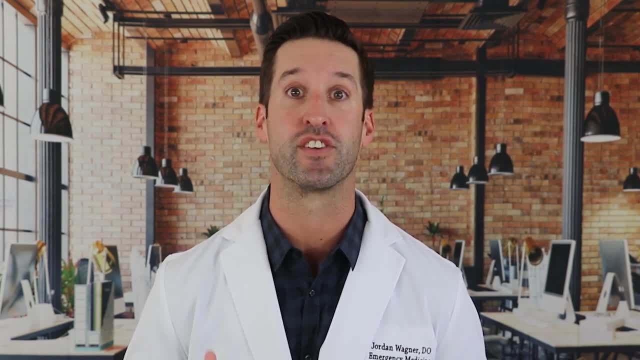 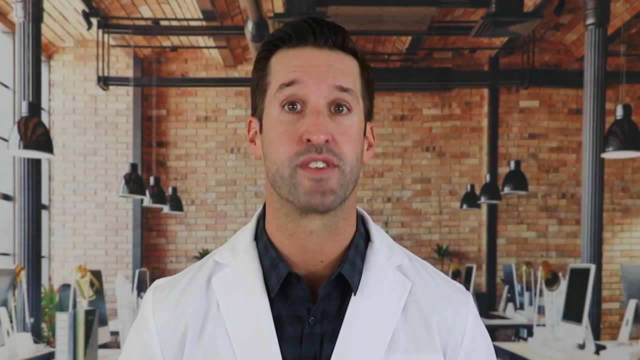 and can send you six feet under when not taken under the direction of a doctor. Do performance-enhancing drugs boost performance? Some athletes may appear to achieve physical gains from such drugs, but at what cost? It's common sense people. The long-term effects of performance-enhancing drugs. 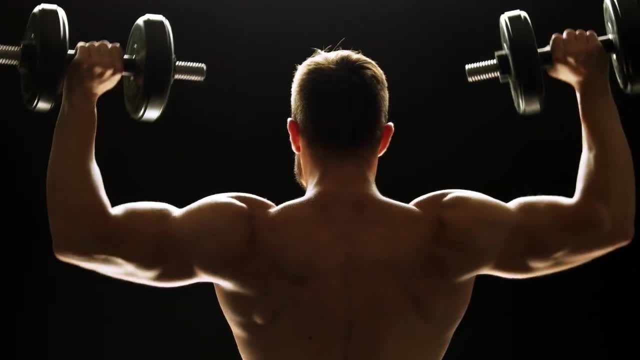 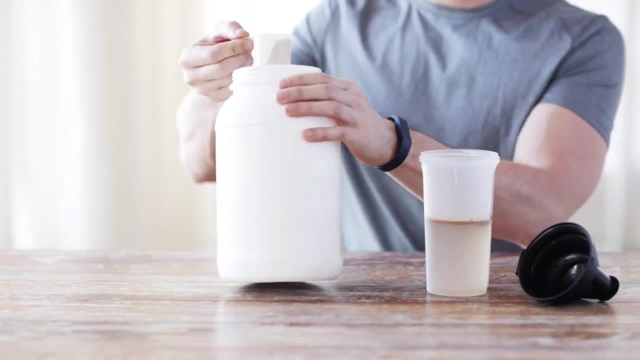 haven't been rigorously studied and short-term benefits are tempered by many risks. No matter how you look at it, using performance-enhancing drugs is a risky business. There are several research-backed supplements which can aid in natural and safe quests for muscle gains. 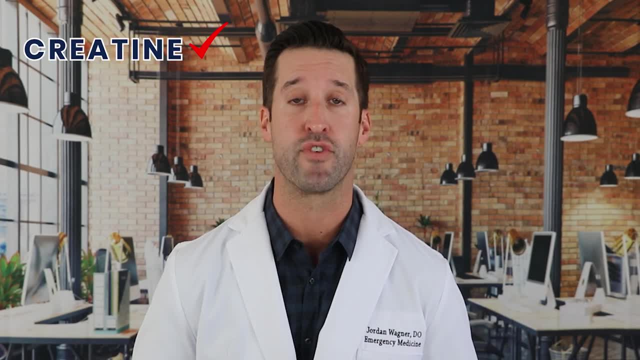 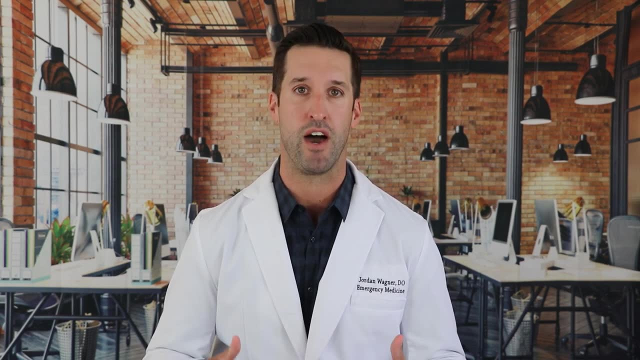 I'd recommend instead checking out supplements such as creatine monohydrate, essential amino acids and whey protein powder. These supplements' safety and effectiveness are backed by a significant, significant amount of scientific research and, by the way, they're legal. 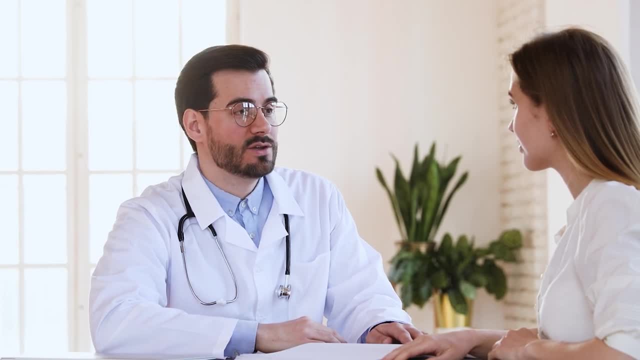 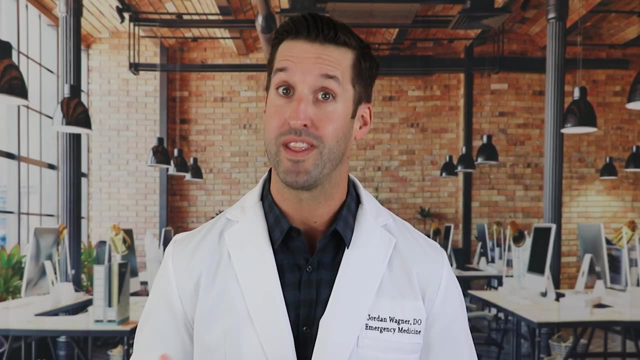 As a reminder, it's always best to run any type of supplement that you want to try by your primary care doctor first. All right, that's been a quick steroid conversation with me, Dr Wagner. Have you or anyone that you've known, 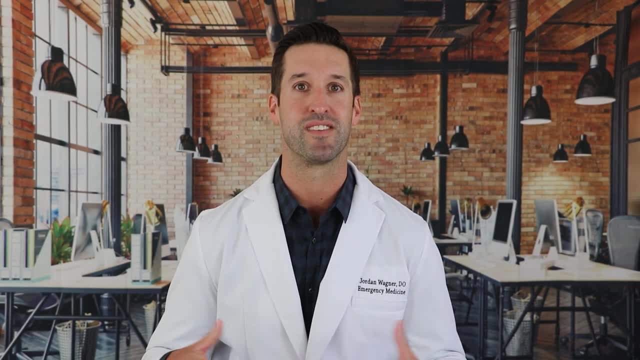 ever taken steroids and experienced any of these side effects? Please let me know in the comments. And also let me know if there are any other medical questions that you would like me to answer. I'd love to hear them Also. please make sure you subscribe and turn. 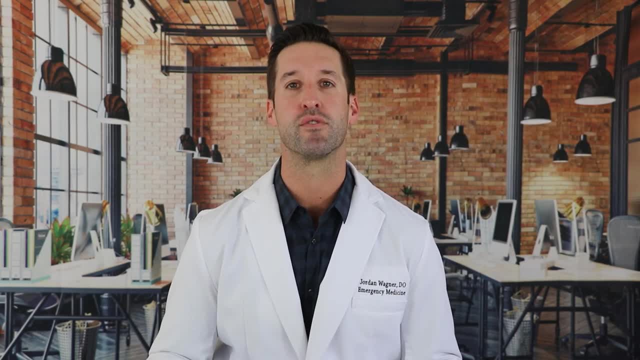 on the notification bell. When you do that and you hit that like button, you let YouTube know that you'd like to see more videos like this one. Thank you so much for watching, and stay healthy, my friends.